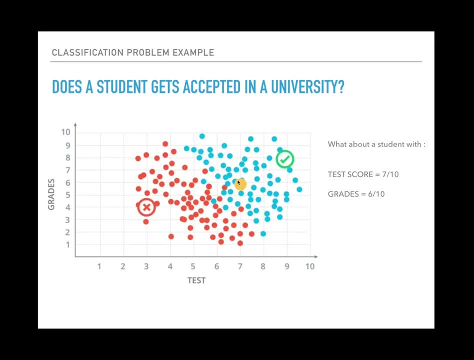 around here, Yeah, So he will lie around here and I think he might get accepted. So we want to form a boundary line, a linear line which will divide the blue points and the red points and a few misclassified points. That is not an issue, That is an error. We have to minimize the error, Not too much. We have to not completely minimize it. 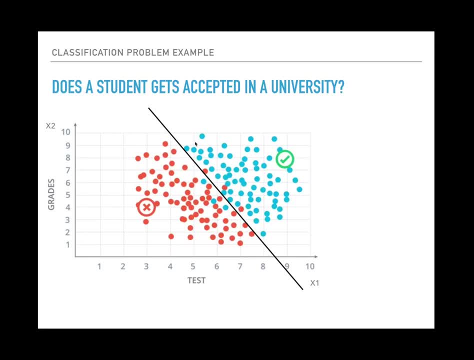 To avoid overfitting of the data. But yeah, that is a complete, completely satisfactory result. So we will find a boundary line that is W1, X1, W2, X2 plus C. Now C is a constant, We can say it as a bias- And W1, W2 are the weights And X1 and X2 are the parameters we input into our test and grade scores So we can calculate the score. 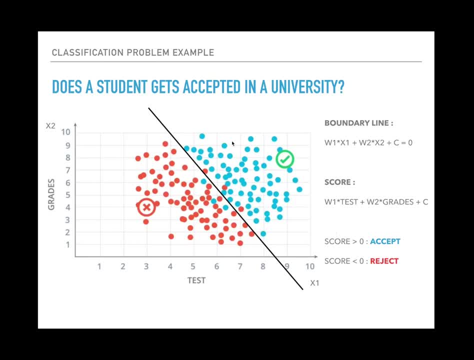 Out of this, And if the score is greater than zero, that means the point lies in this region. So the student gets accepted, If it is less than zero, it gets rejected. Pretty simple. Now we can also say the boundary line as WX plus B in the form of matrices. So we can say it as a 1 cross 2 matrix and a 2 cross 1 matrix of matrix. So if you multiply it we can get a 1 cross 1.. 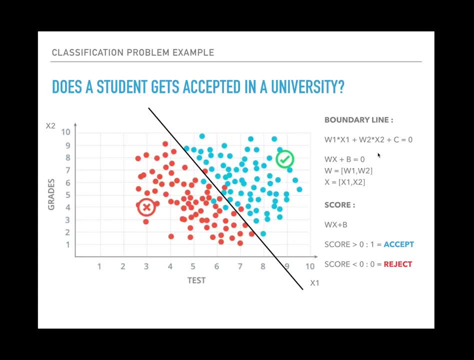 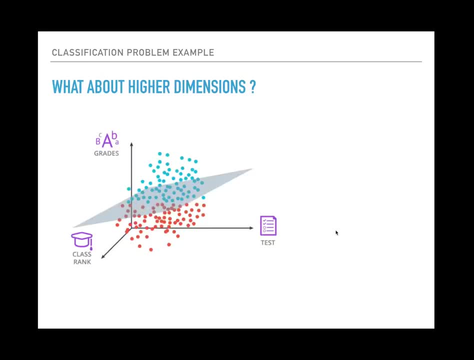 Value And we add the bias to it, So we can form a boundary line in the form of matrices. Same thing, Nothing. Now what about higher dimension? Say, the university accepts class rank also. So we will form a 3D plane. 3D And a plane would divide the blue points and the red points, And we can form three parameters: W1, W2, W3.. And X1, X2 and X3 would be our. 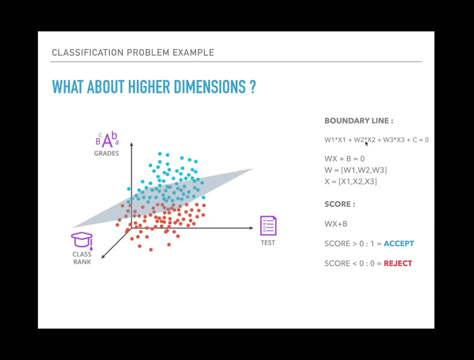 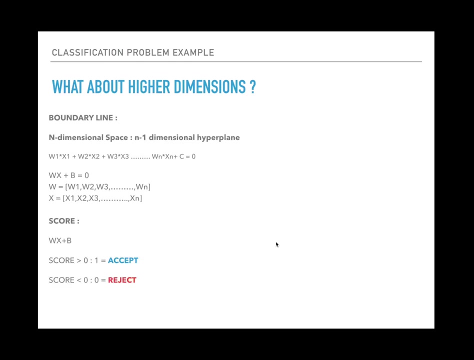 Input values. So again same equation. we will form WX plus B And same score, Score greater than zero. We say the label as 1.. Xn less than zero, Zero will label And reject. So what about if there are n dimensional space, n parameters? So what we will form? We will form an n minus 1 dimensional hyperplane, basically. So we cannot visualize it. 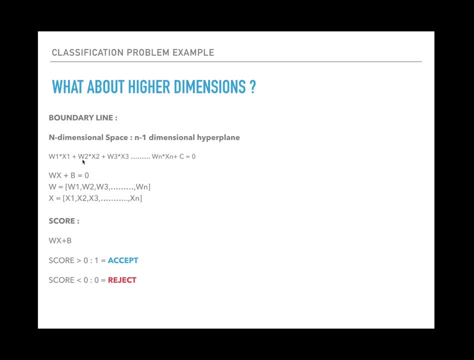 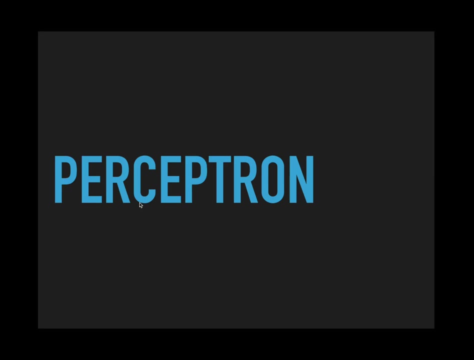 So we have written the equation here. So W1 plus X1.. W1 into X1.. W2 into X2.. W3 into X3. And dot, dot, dot, Wn into Xn plus some bias. So same equation: Wx plus B. Now this time it is 1 cross n into n, cross 1 matrices. Same score, Same thing. But we cannot visualize this dimensional hyperplane. So perceptron algorithm. So what it does is In this same example. we will take the scenario. 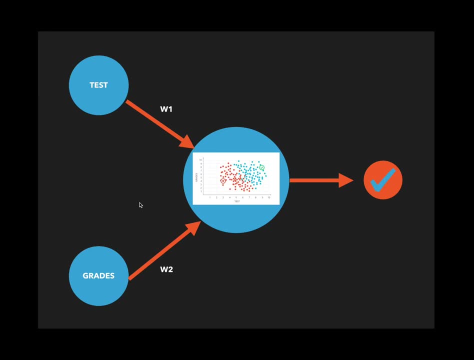 So what perceptron wants is a test and grades. We will assign some weights to it And calculate, Get some calculation and assign if the student gets accepted or not, Basically the boundary line. Now, what we did was calculate the score WX plus B. Now, why not? we assign the B as input. only We can. 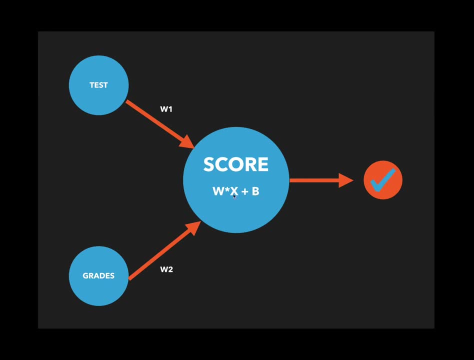 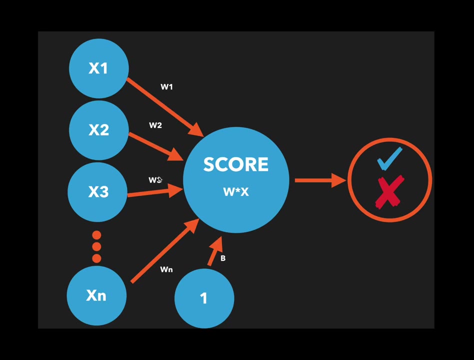 one as the input and B as another weight. and if there are any inputs, we can take n inputs, w1, w2, w3, wn would be the n weights and B as one of the biases, as one taking the input. okay, and we could calculate the score and decide if the 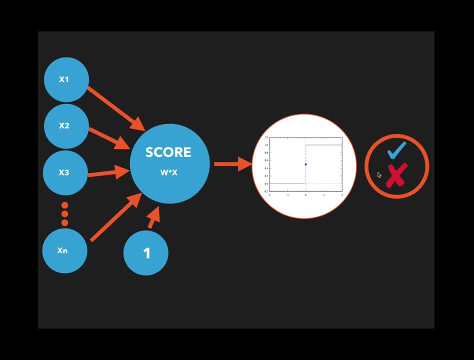 student gets accepted or not. now another thing. now what we have to do is we assign the labels 1 or z, one and zero. we can calculate the labels tools by the step function. if the values, the score, is greater than zero, we can say of the step. 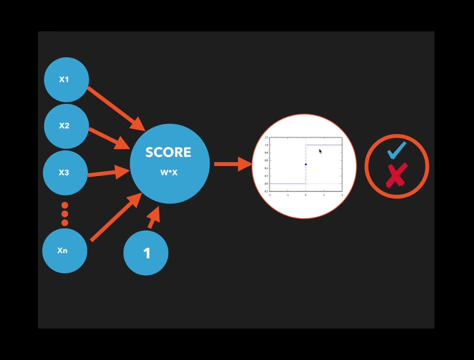 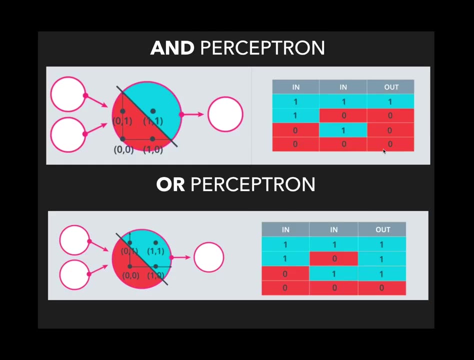 function would give one. if it is less than zero, it would give zero. so one label would say the student gets accepted. 0 would say rejected. now perceptron are of. we can see the two types of perceptron and perceptron and or perceptron. there is a. 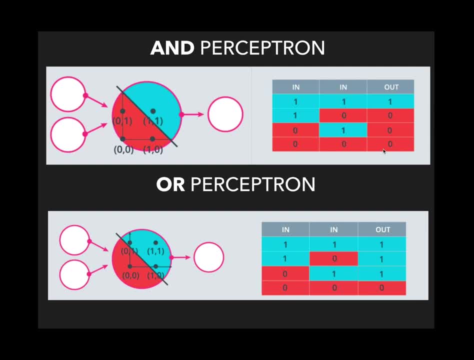 other perceptrons also. so what an and perceptron is? basically there are a few points: 0 comma 1, 1 comma 1, 1 comma 0, 0 comma 0 now, and perceptron would draw lines like this and it would accept 1 comma 1, 1 comma 1 and reject all these.